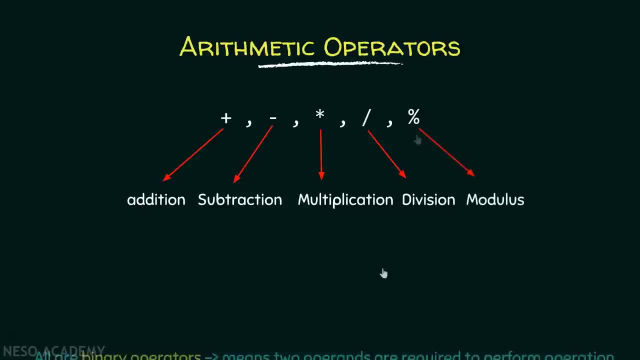 And the last one is called modulus operator. Apart from this thing, all are binary operators, Means two operands are required to perform operation Right. For example like: if we want to perform the addition, then we are always performing addition between two numbers. 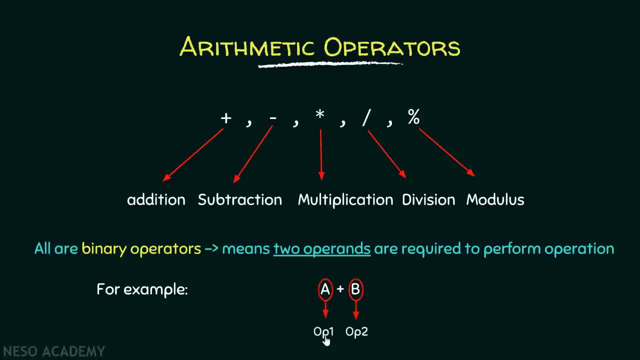 This one is the first operand and this one is the second operand: OP1, OP2.. OP simply means operand. Okay, If we want to perform addition, we need to have two operands. That is why addition is called binary operator And similarly. 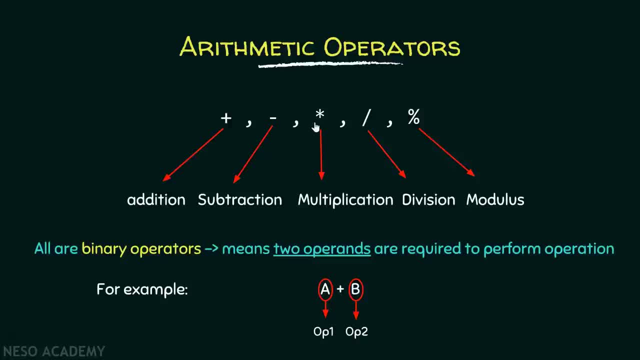 subtraction is also a binary operator, Multiplication is also a binary operator, Division is also a binary operator And modulus is also a binary operator. Now let's consider one example. Here you can see I have declared two variables, a and b. 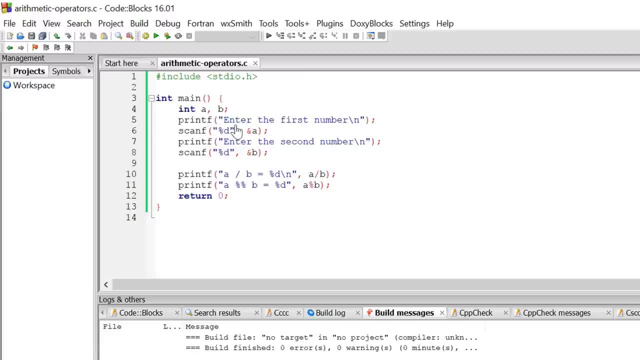 With the help of this printf function, I would be able to ask the user: please enter the first number. With the help of this scanf function, I would be able to accept input from the user. With the help of this printf function, I would be able to ask the user. 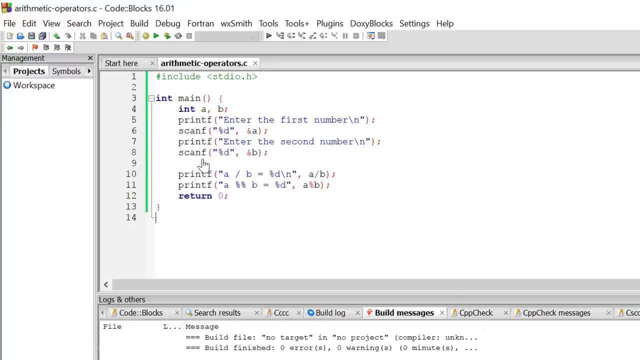 please enter the second number. With the help of this scanf function, I would be able to accept the second input from the user. I am simply going to print the result of division as well as the modulus. Division will result the quotient and modulus will result the remainder. 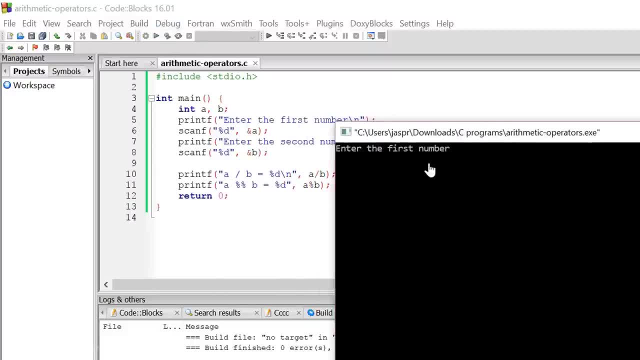 Let's execute the code. Suppose I enter nine as the first number, then I enter three as the second number, then this would be the result: Result of division of these two numbers, nine and three. that is, when nine is divided by three. this gives us the result as: 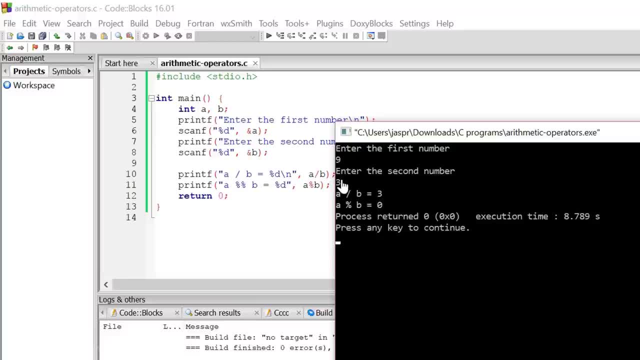 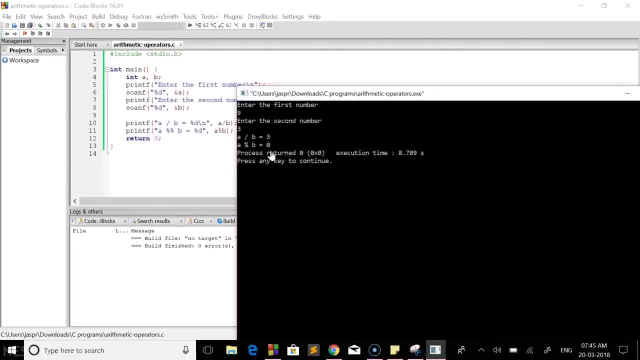 three, which is the quotient, And when nine is divided by three, the remainder would be equal to zero, And we know this thing already, So there is no problem in understanding this concept. Okay, Now let's talk about the precedence of operators and associativity. 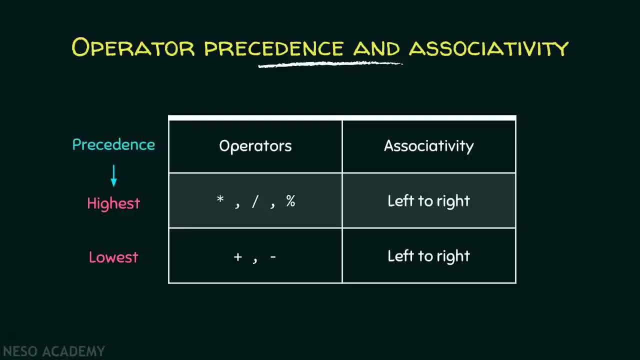 Suppose you have an expression like a plus b into c, divide d. Precedence simply means that which operation is going to perform first in that expression and which is going to perform last. Here you can see multiplication, division and modulus. all are having the same precedence. 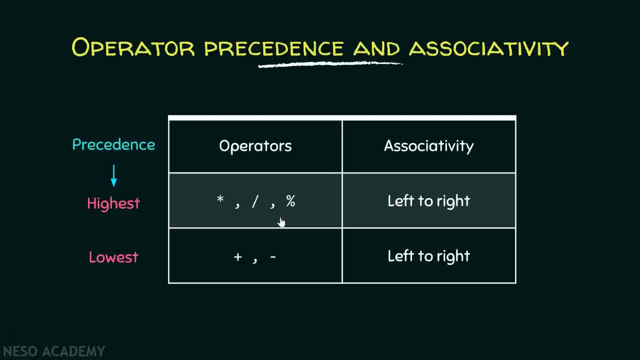 If suppose these operators are there in your expression, then all are having same precedence. It is not the case that division is going to perform first, then multiplication and then modulus. All are having same precedence. On the other hand, when we have addition and subtraction, then these two 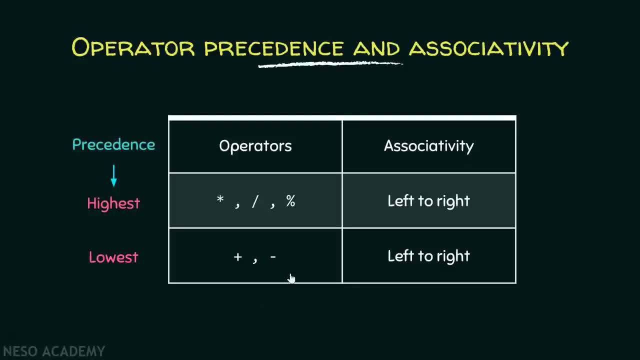 operations are also having same precedence. Suppose we have an expression like a plus b minus c, then we cannot say that subtraction is going to perform first and then addition. They both are having same precedence. Now one important point. Suppose we have an expression like: 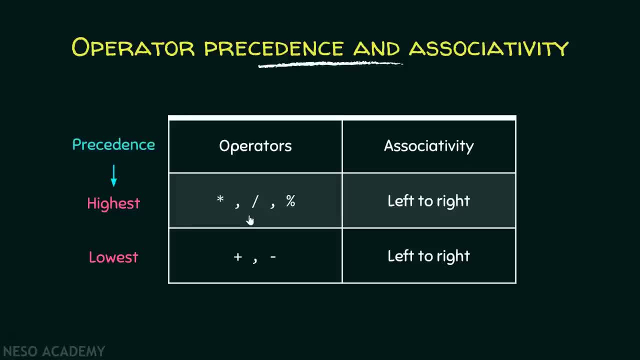 a divide b plus c. In that case the division is performed first and then the addition. That means a divide b is performed first and then the addition, Because precedence of this set is highest and the precedence of this set is the lowest. Multiplication, division and modulus. 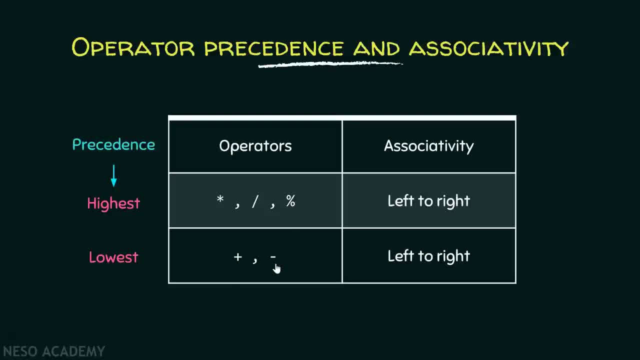 is performed first in the expression, and then addition and subtraction. Now, as we know these things, suppose in our expression we have multiplication, division and modulus. only, As we know this thing, that the precedence of these operators are the same. Now, in that case, which is going to perform? 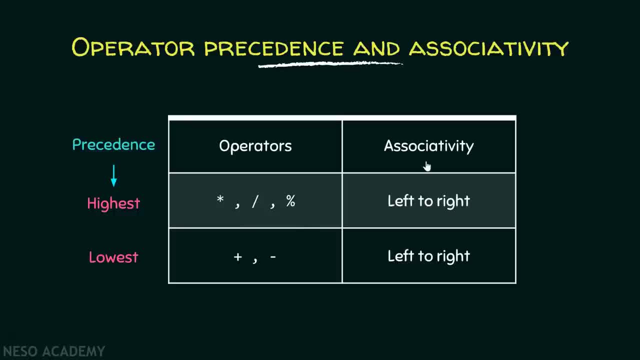 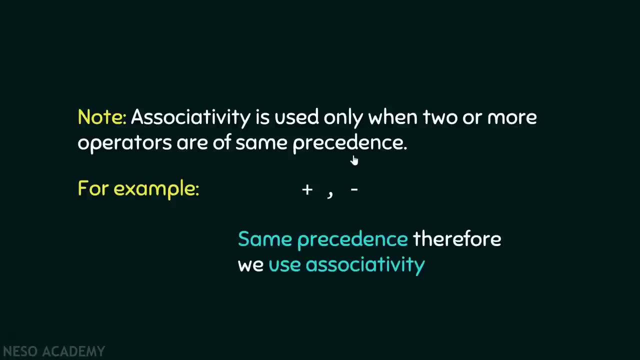 first, If precedence of operators are same, then associativity came into picture. Associativity for these operators are from left to right and for these operators also from left to right. Associativity is used only when two or more operators are of same precedence. 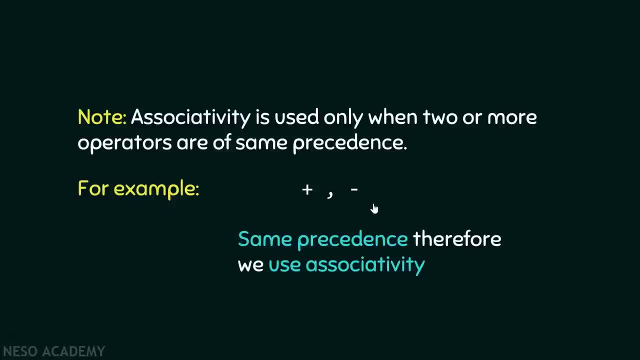 For example, we have plus and minus right. These two operators we know have same precedence. Therefore we use associativity, That is from left to right. Suppose we have an expression like a plus b minus c. In that case the addition is going to: 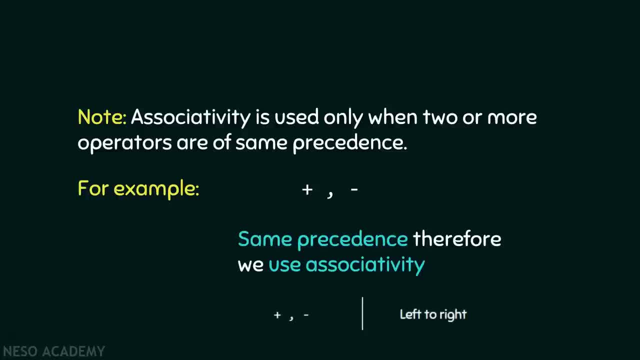 perform first because it is in the leftmost side, And we know this thing: associativity for addition and subtraction is from left to right. Therefore, the leftmost symbol, which is addition, is going to perform first and then the subtraction. Now let's consider one coding example. 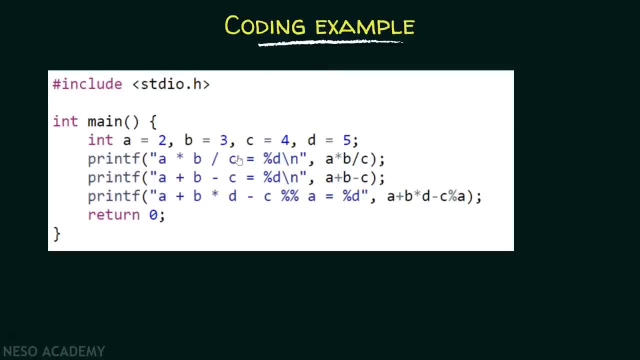 Here you can see, I have declared four variables- a, b, c and d, And I assign them values two, three, four and five respectively. right In this printf function. I am trying to print this expression along with the result of this expression. 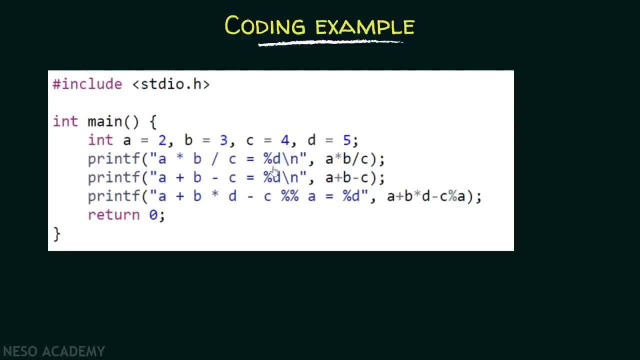 which is a into b divided by c, This percentile d is going to get replaced by the result of this expression. Similarly, this percentile d is going to get replaced by the result of this expression. And this percentile d is going to get replaced by the result of this. 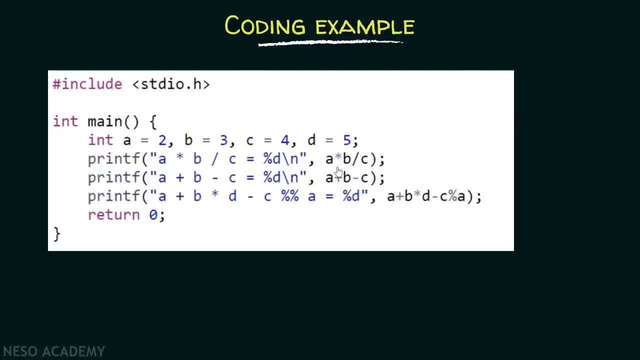 expression. If we evaluate this expression a into b divided by c, then this is equivalent to two into three divided by four. As you know this thing that multiplication and division are having same precedence. Therefore, associativity came into picture, and associativity of multiplication. 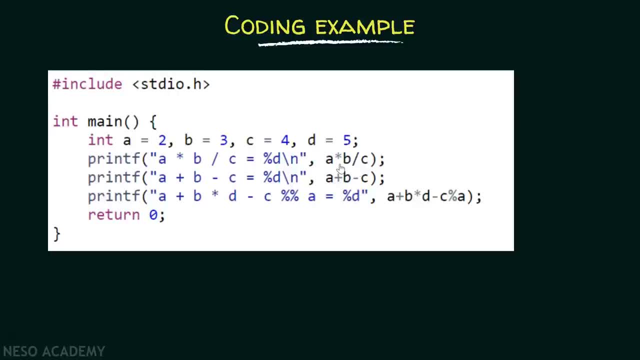 division and modulus is from left to right, Right. Therefore multiplication is going to perform first and then the division a into b is going to get evaluated first. that means two into three, which is equal to six, And six divided by four, which is equal to one point five. 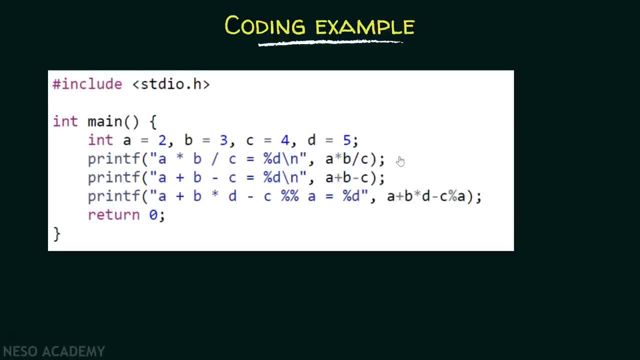 As we are trying to print an integer, therefore, that decimal part is truncated and the result is one. For this expression also, we know this thing: that addition is going to perform first and then the subtraction, Because they are having same precedence and associativity is from left to right. 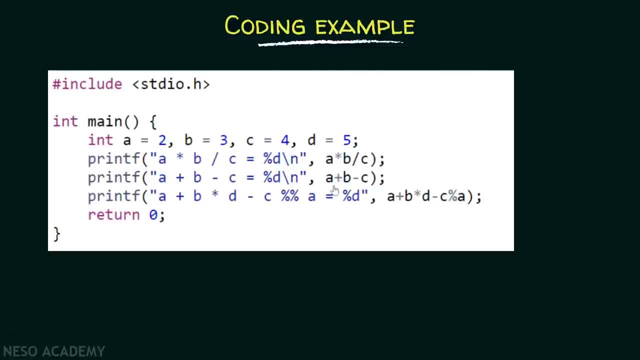 Therefore, addition is performed first, and then subtraction: a plus b, which is equal to two plus three, that is equal to five, and c is equal to four. Therefore, this printf function will also print one. In third printf function we need to know two things. 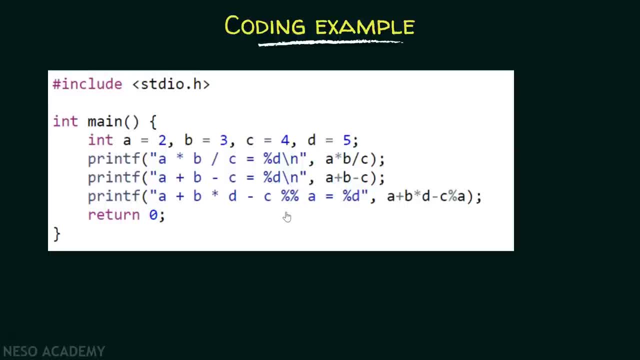 First of all, I put two percentiles here because I need to print one percentile onto the screen. If you simply write one percentile, then compiler would think of percentile a as a format specifier, which is not what we want. Therefore, to eliminate the confusion, 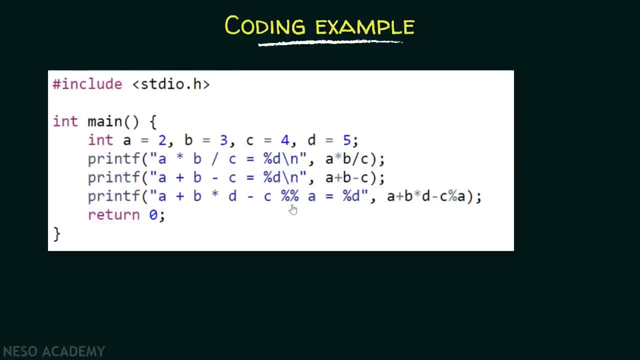 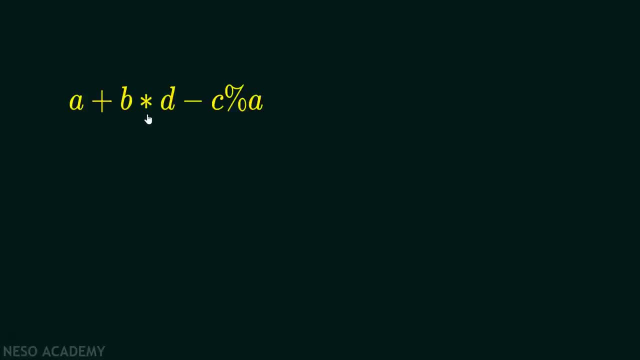 we are putting two percentiles to print one percentile onto the screen. Okay, Let's evaluate this expression. This is our expression. We know this thing: that multiplication and modulus are having higher precedence as compared to the addition and subtraction. Therefore, they are going to perform first. 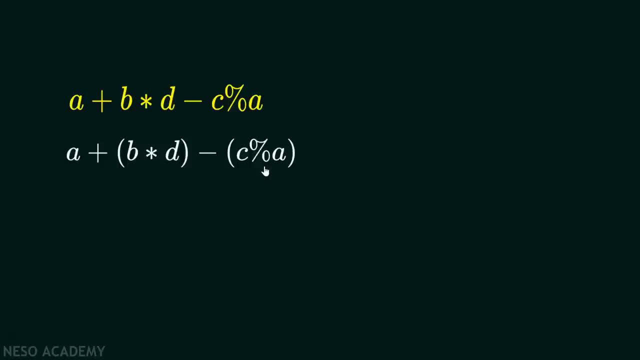 This bracket simply means that multiplication and modulus is going to perform first as compared to the addition and subtraction. After replacing the values, this expression looks like this: a plus three into five minus four mod two, Three into five is equal to fifteen and four mod two is equal to zero.